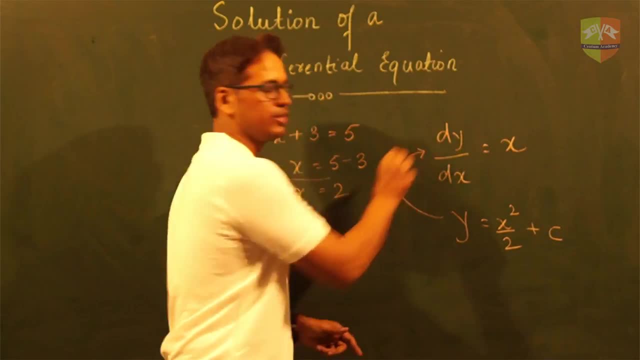 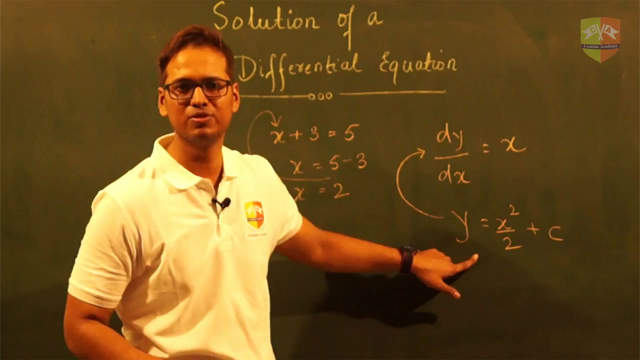 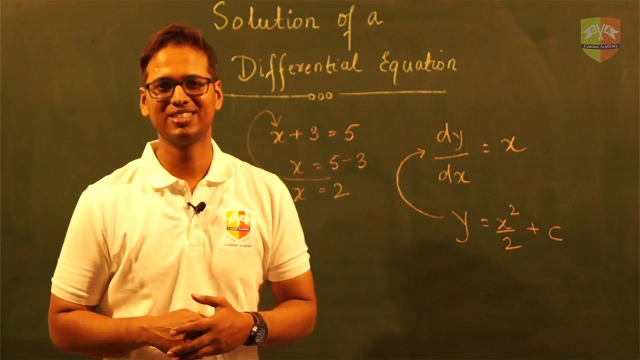 So this is a solution for this differential equation, Or, in other words, this differential equation has been formed from this family of curves. right Now, to tell you frankly, while you were doing integration chapter, you were actually already learning how to find solutions for differential equation, right? 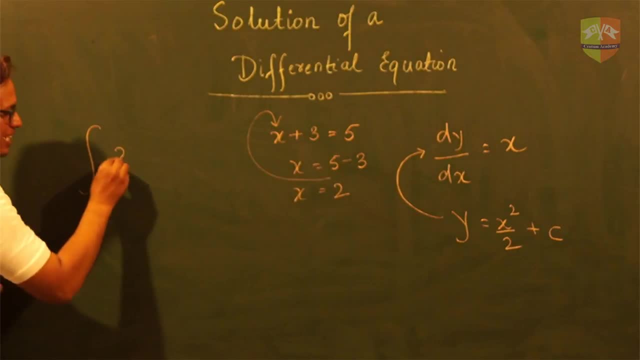 So when a question like this was posed to you, what is the integral of, let's say, 2x plus 5 with respect to dx, right? And you integrated the answer to be x square plus 5x plus c, right? 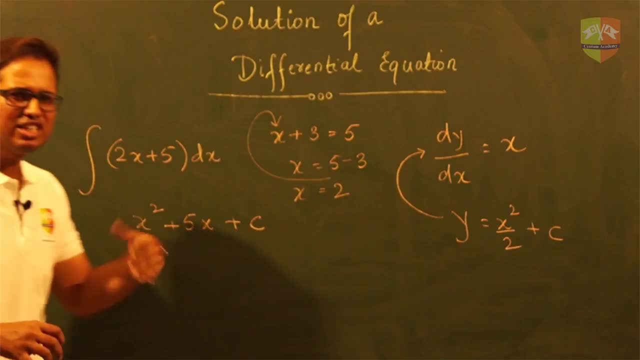 The same thing. if I have to write in the form of a differential equation, I would say: what is that curve? What is that curve whose derivative gives you 2x plus 5.. So your answer will be: the curve whose derivative gives me 2x plus 5 is nothing but. 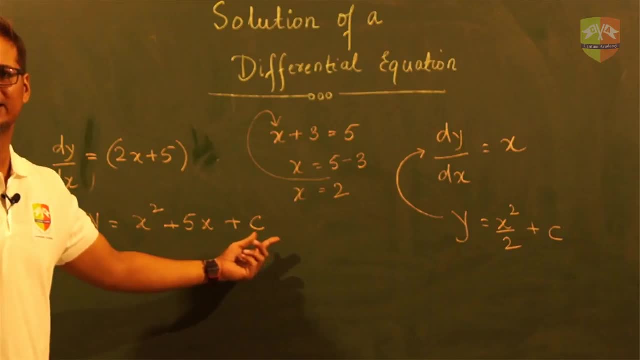 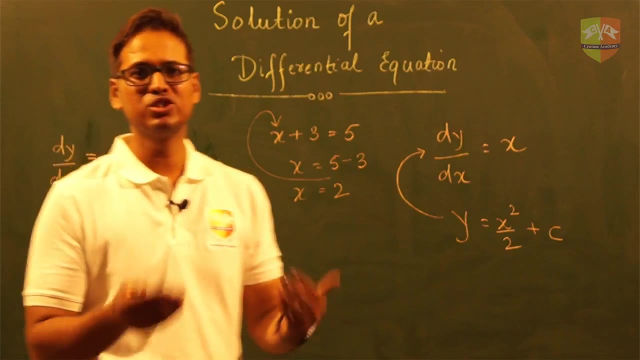 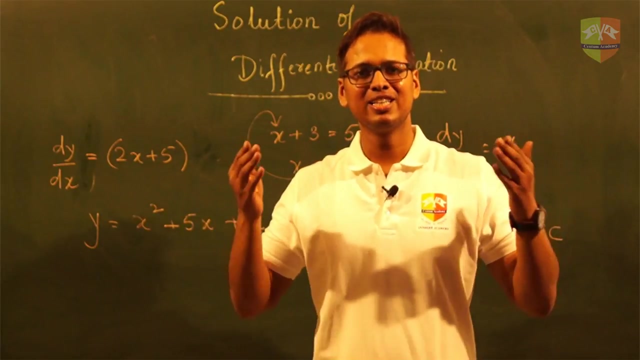 y equal to x square plus 5x plus c right, Where c is an arbitrary constant. So indirectly you are actually learning how to find solutions of differential equation. So whole integration chapter was nothing but solving or finding the solutions for differential equation of order 1, right. 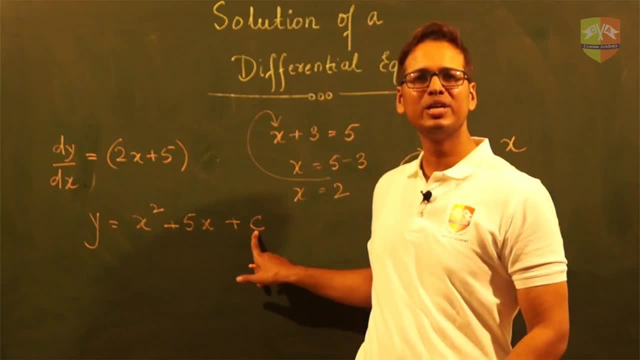 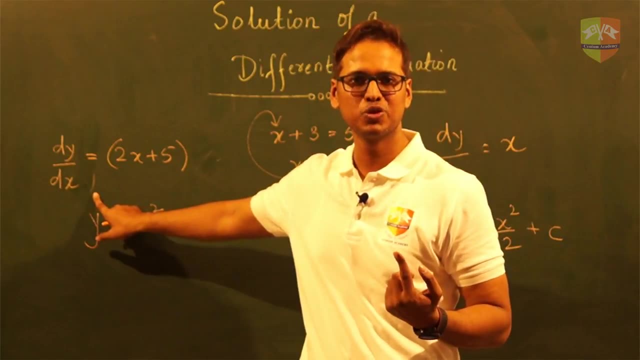 How do we know it's order 1?? Because ultimately we are going to write c, one arbitrary constant involved, And in other words we have only dy by dx term. So the highest differential coefficient occurring in that particular differential equation is 1.. 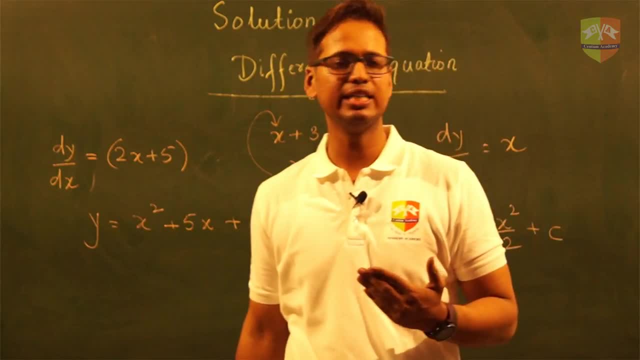 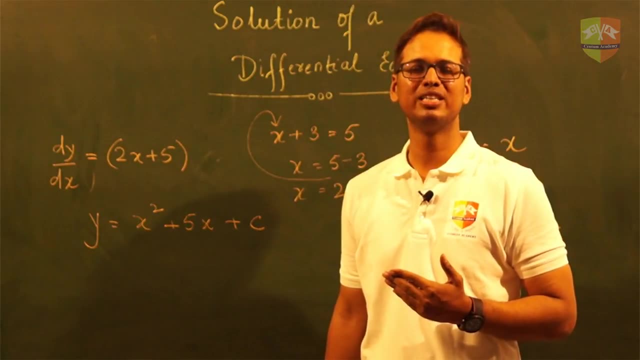 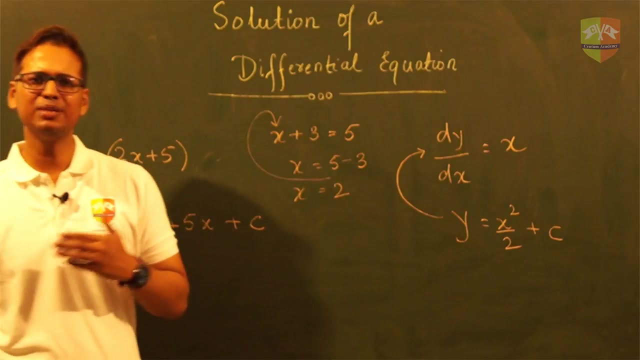 So in the integration chapter, particularly indefinite integration, we were learning how to solve differential equations of order 1. Or we were learning the solutions for that, Okay, Okay. So in this video, my main aim is to tell you how many types of solutions are there for the differential equation. 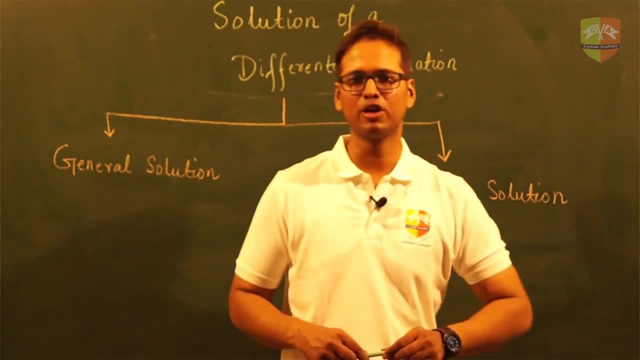 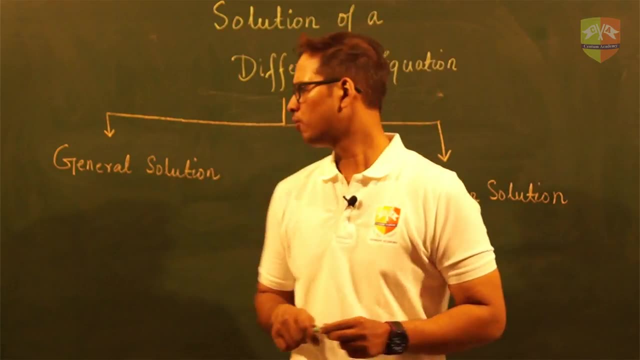 Alright, Now talking about the type of solutions possible for a differential equation. Normally we speak of the solution to a differential equation are of two types. One is called the general solution And the other one is called the particular solution, Right? 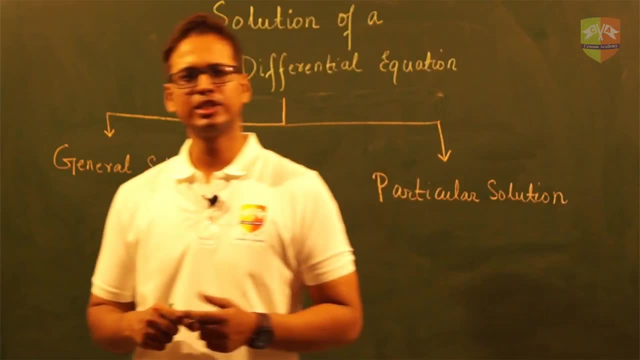 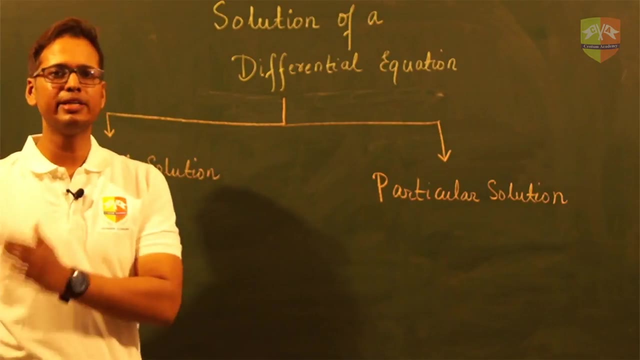 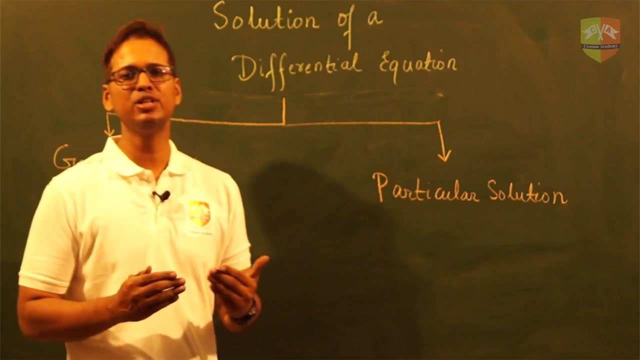 Now, what is a general solution? To explain you in words, general solution of a differential equation is that a family of curves which contains the arbitrary constants. right, But however, if you involve some values or if you assign the values to those arbitrary constants, 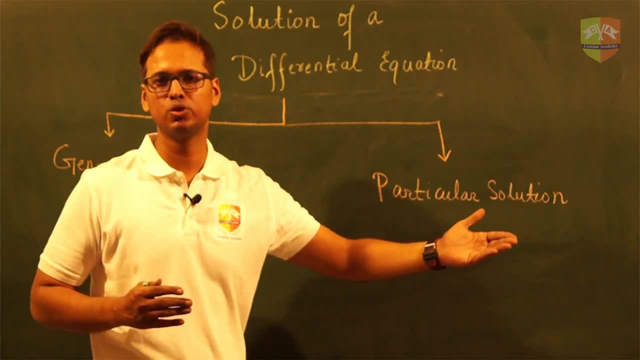 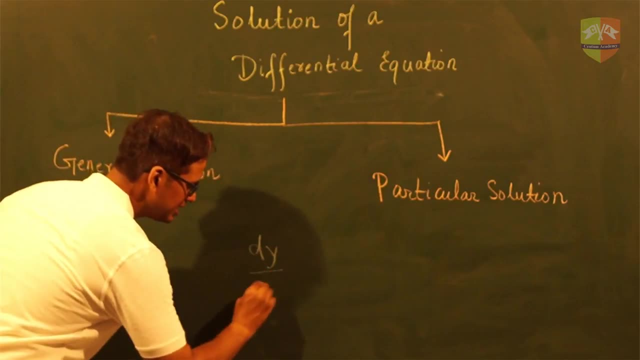 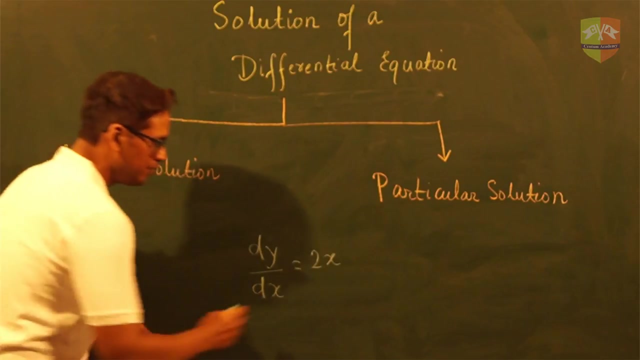 that general solution will convert itself to a particular solution, Right? Let me explain this with the help of an example. If I say dy by dx is equal to 2x, Right? So when we solve this differential equation, we solve this differential equation as: 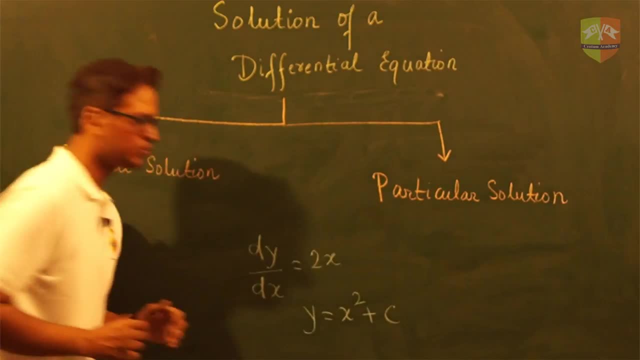 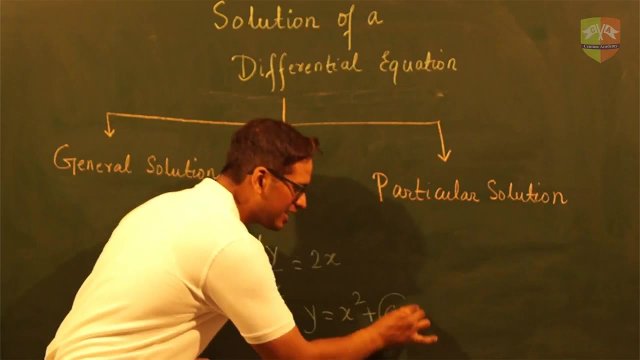 or y equal to x square plus c. So y equal to x square plus c is a solution for this differential equation. Now, because I have written a c here, which is an arbitrary constant, and I don't know what is the value of this arbitrary constant. 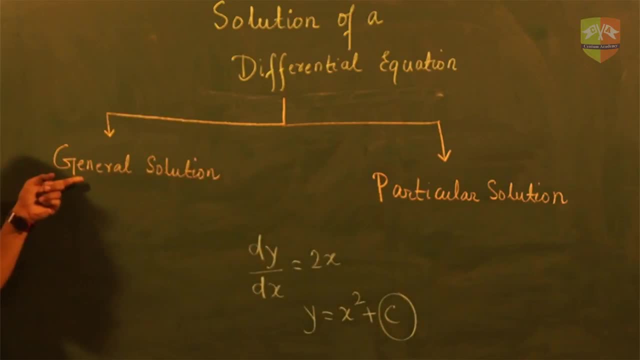 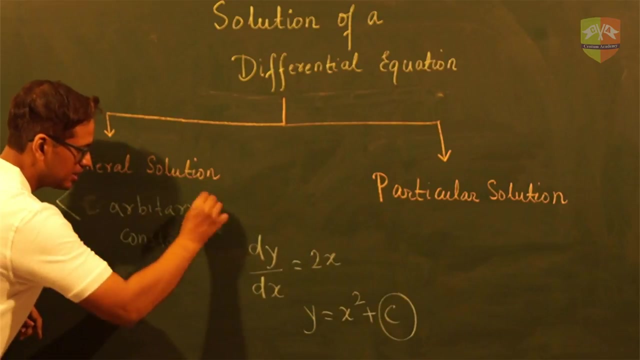 such a solution will be called the general solution, Right? So in short, in the general solution c or arbitrary constants, we can say arbitrary constants would be present, So it would contain your arbitrary constants, Right? That depends. what is the order of that differential equation? 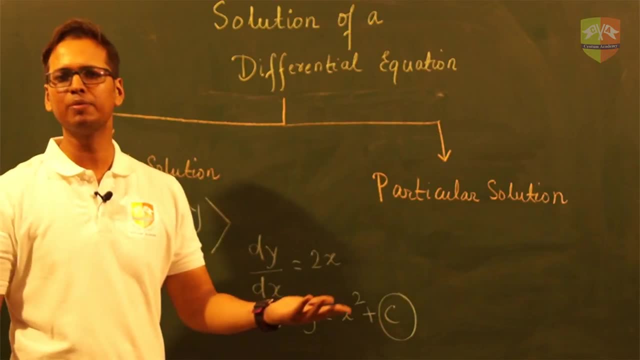 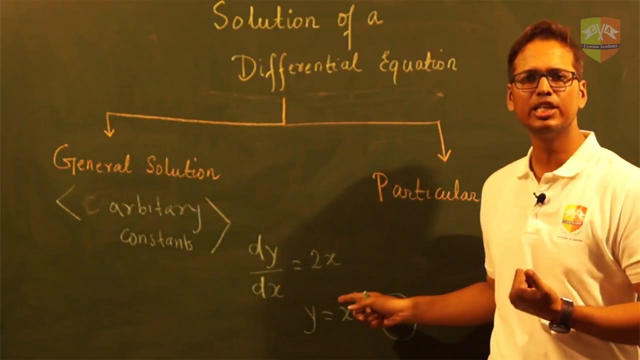 So if it is a second order differential equation, it will contain two arbitrary constants. If it is a third order differential equation, it will contain three arbitrary constants. So since this is an order one differential equation, it will contain one arbitrary constant. 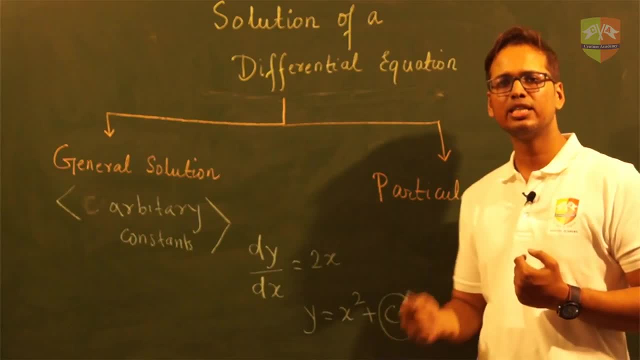 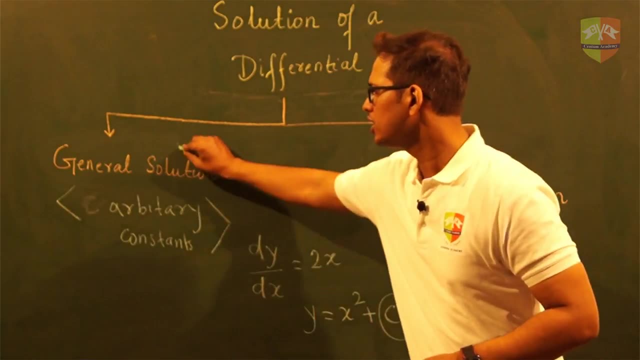 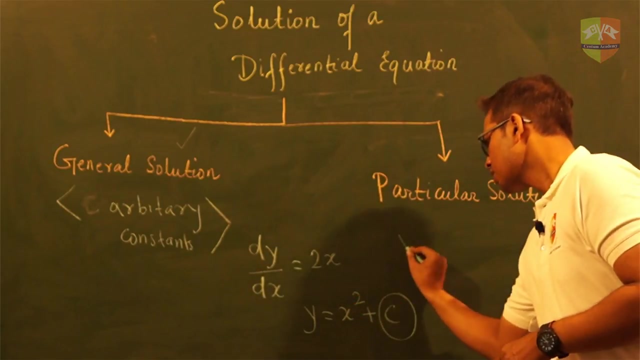 So writing a solution where an arbitrary constant is written and I don't know what is the value of that arbitrary constant, then that solution will be called the general solution. On the other hand, the very same differential equation: if I say y is equal to 1 when x is equal to 0. 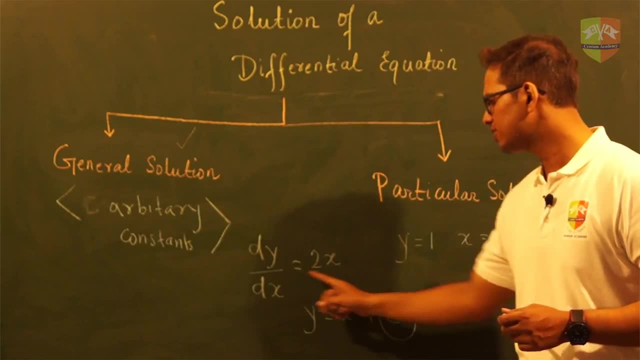 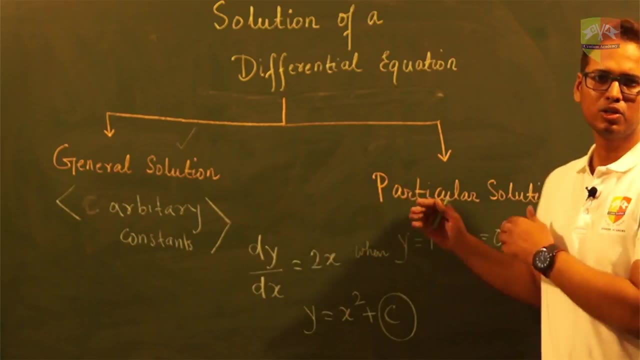 Right. So find the solution for this differential equation when y is equal to 1 and x is equal to 0. Then, in order to find the solution, we will say: the general solution is y equal to x. So the general solution is y equal to x square plus c. 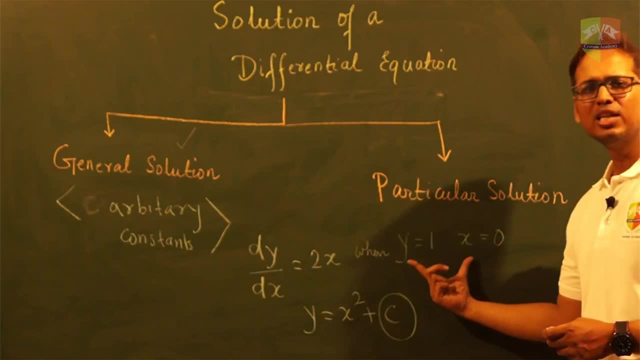 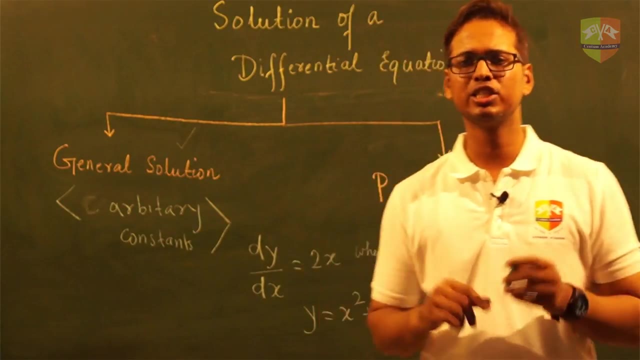 No doubt about that. And then we will use this value. This value is called the initial values Right. Normally in the terms of differential equation chapter we call such information given to us as initial values, So these are called initial values.